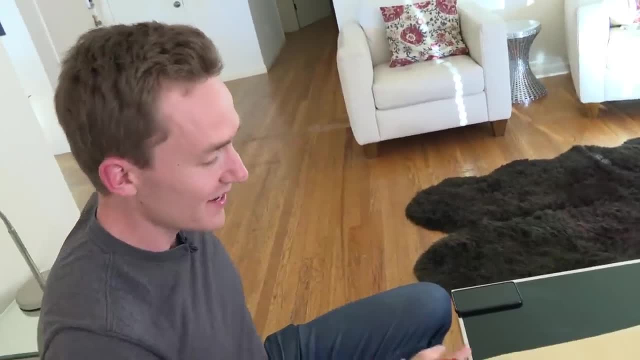 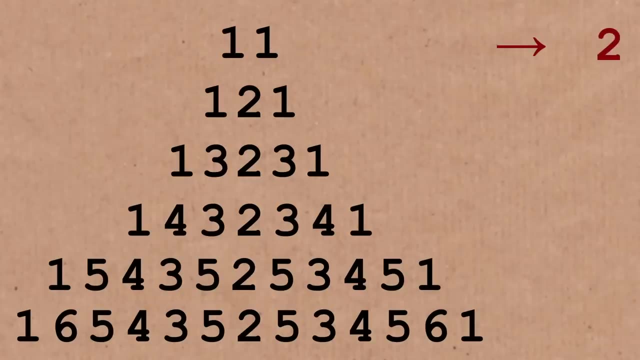 are the patterns I can observe in this Pascal-esque pyramid, and if they just count how many elements are there in each row, they'd say: this one has two numbers in its row, this one has three numbers, this one here has five numbers, seven, eleven, thirteen, and so you're compelled to ask: okay, how? 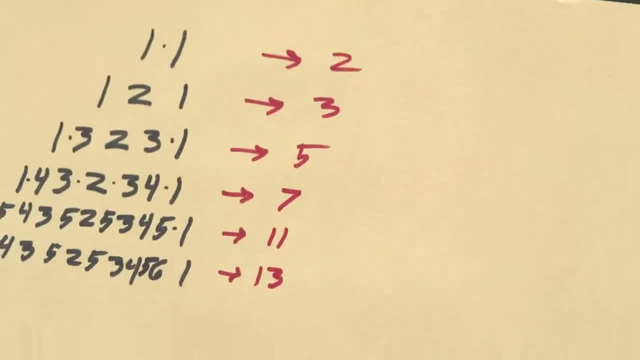 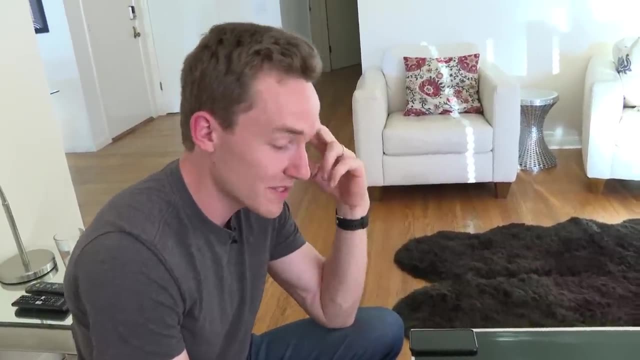 is this numbers? Yeah, and um, you know I could say, is there any reason that we should expect prime numbers from this? You know, is this is just a completely random tower? you know, is there any reason we might expect prime numbers? and I could say, actually this isn't as random a tower as you might think, It's related. 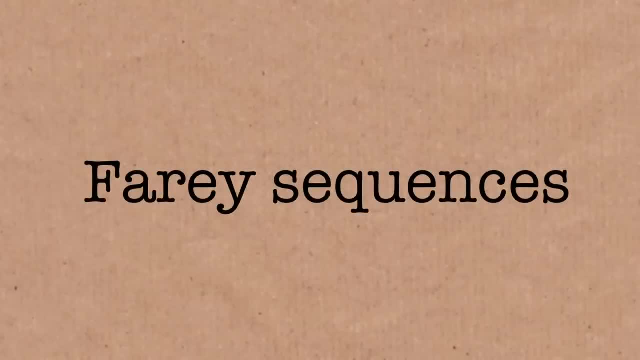 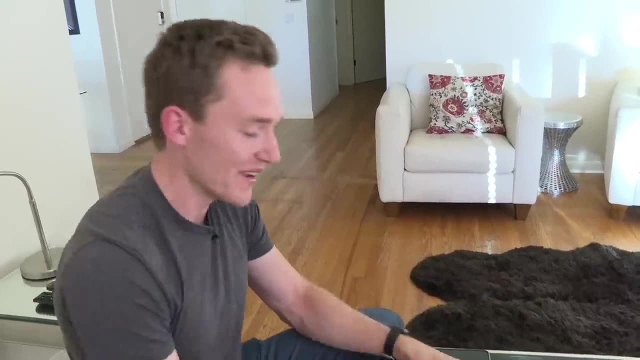 to these things called fairy sequences, where, if I want to write out what are all of the rational numbers where the biggest possible denominator is 1, that sits somewhere in the interval from 0 to 1, there's really only two rational numbers available. I can have 0, which I could write as 0 over 1. 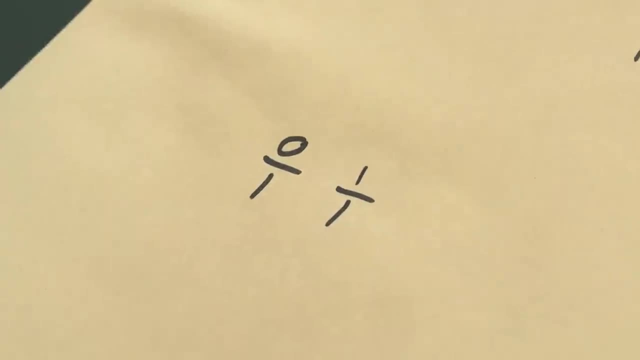 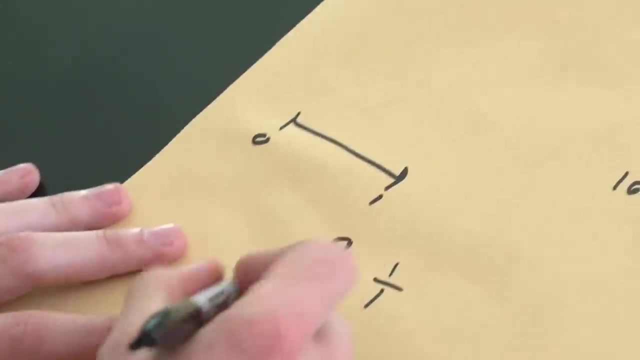 or 1, which is 1.. 1 over 1, and if I say, okay, what are all the rational numbers in that interval? you know kind of the unit interval from 0 up to 1, with a denominator that is at most 2, and you could say: well, I've got those, those two that I already had, but I 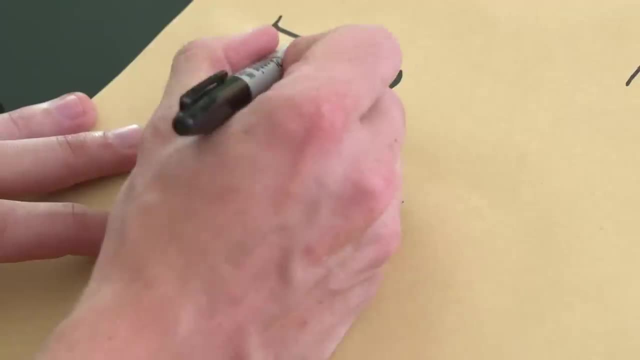 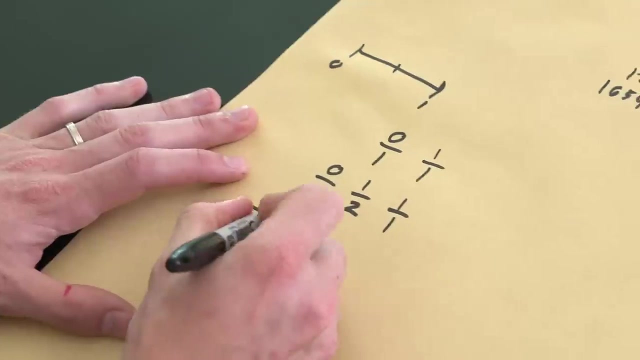 now could also include 1, half into those, and so you know, kind of might mark a half, and what if we allow the denominator to get as big as 3 and you say, well, in that case I can have all of the ones that I previously had, but also 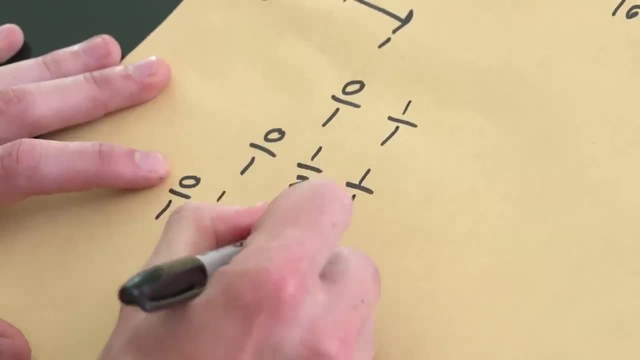 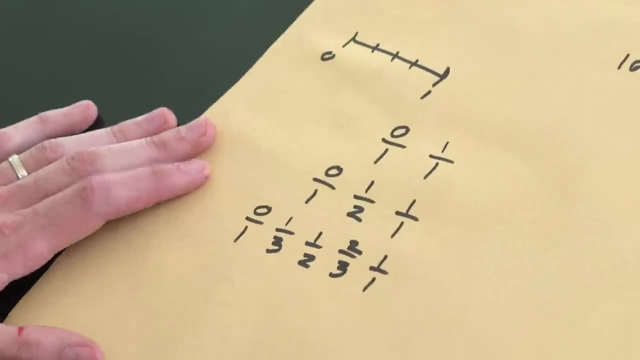 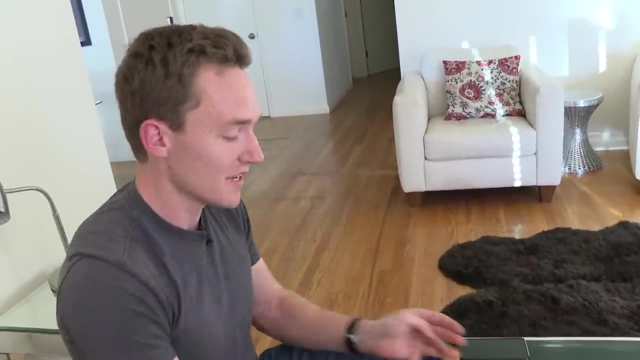 a third is available and a half, and also two thirds is available, and I'm writing them in the order that they would show up on the number line, so I'm kind of sorting them from least to biggest. you can show, actually, that this sequence here, of this very sequence, all of the rational numbers maximized by a certain 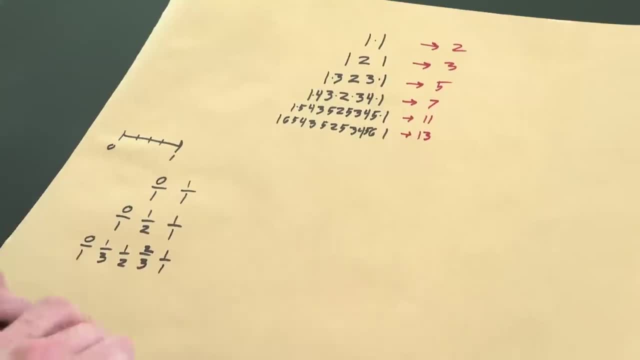 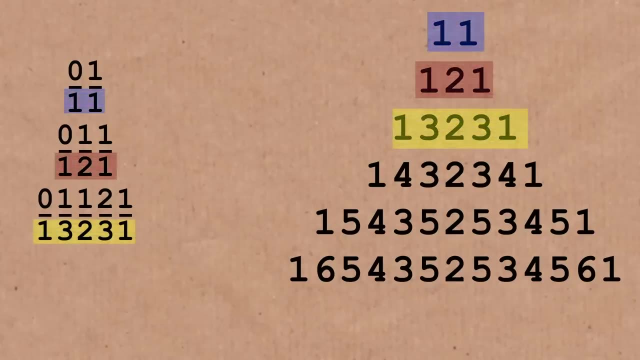 denominator is exactly the same as what we were doing up here. all of the denominators on the bottom correspond to one of the rows up here, and there's a kind of cute reason for it. or when you have a sequence of three different rational numbers in this very sequence. so I'll just do one more row. 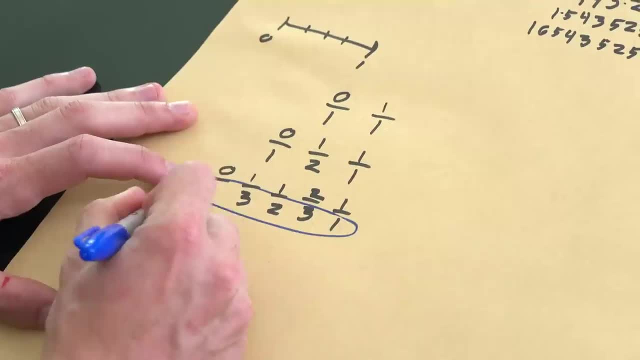 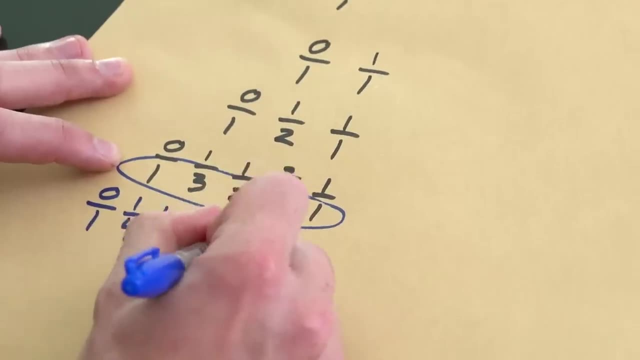 to kind of see, like, where does one fourth or the fourths fit in? we've got 0 over 1. a fourth is going to fit in here between that and a third. then we've got a half, then a third, and then three fourths comes up there and then one. if 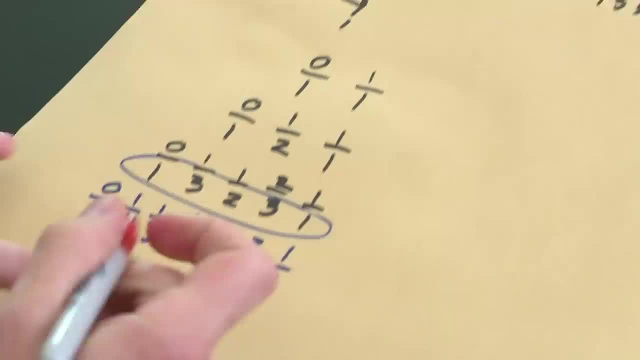 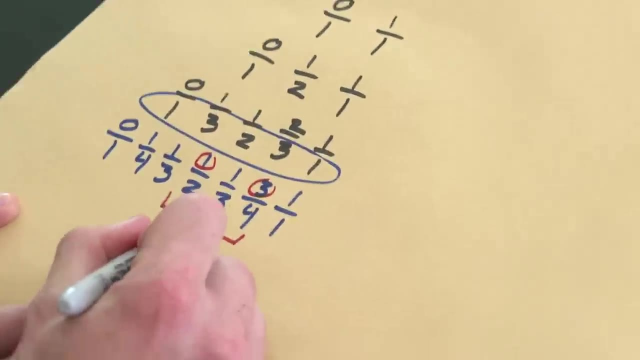 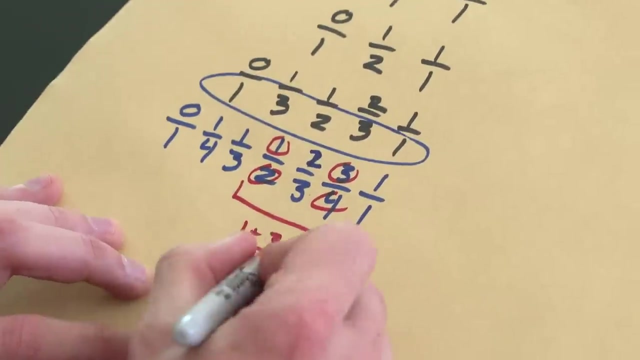 we just look at three adjacent elements, so maybe I take these here. note if I add up the numerators of the two on the outside and then if I add up the denominators also, so I add up the two and the four, two plus four, and I make a fraction out of those. in this case that's the same as 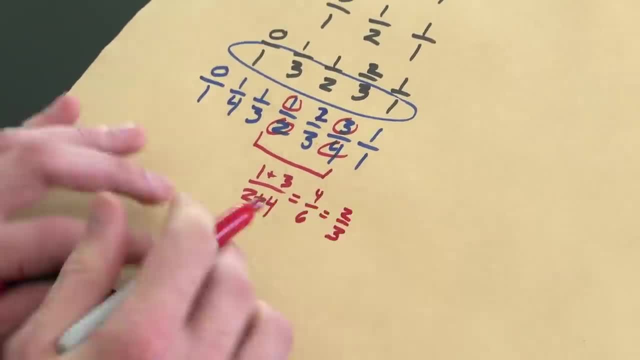 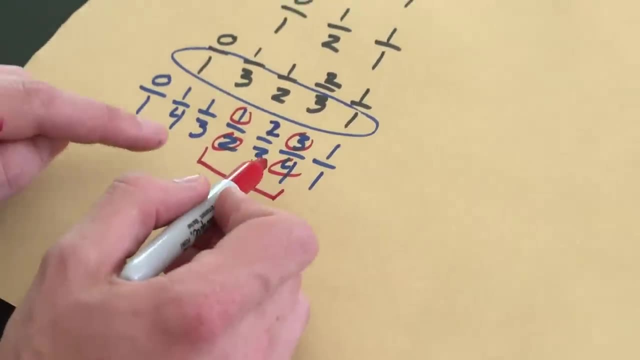 four sixths, which is the same as two thirds. this way of combining rational numbers, where I add the numerators and add the denominator, has a fancy name. it's called the mediant. it's kind of like what a what someone who hasn't yet learned about fractions might think you do and you're supposed to add two. 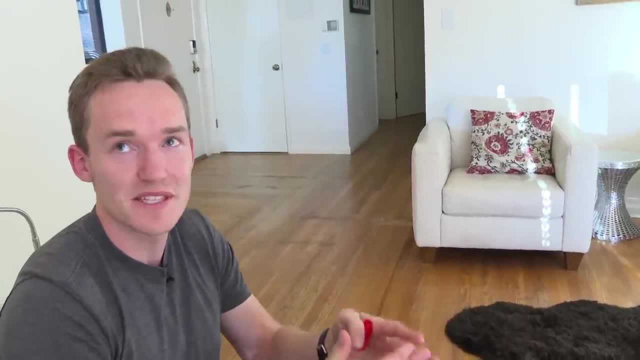 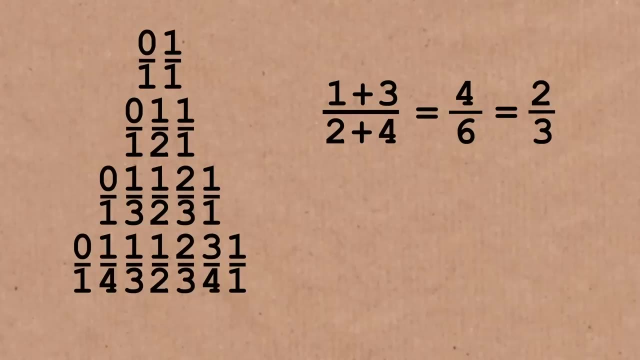 fractions. it's not a wholly useless operation. it always gives you something that's between those two and in fact in these fairy sequences it'll always be the case that the mediant of two that are offset gives you the one that sits in between. you can kind of see the connection between this in the pyramid. 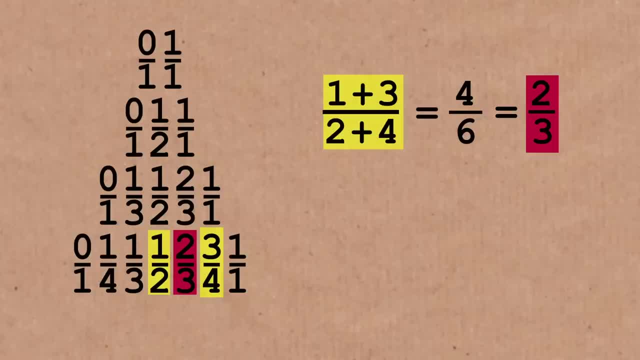 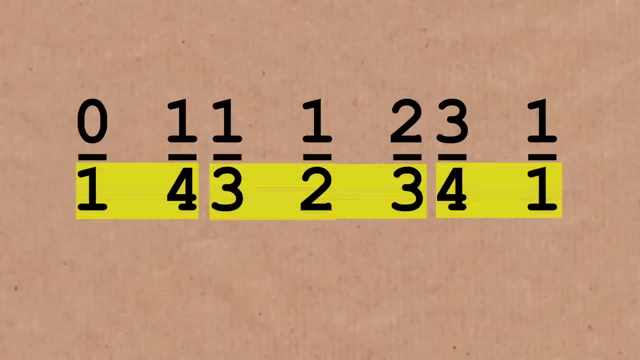 because you need the denominators to add up. so every time you're squishing in you say, hey, I'm gonna introduce the possibility that five is a denominator. the only way that that could happen is if it's two neighbors had denominators that added up to five. so you look in the previous sequence that corresponds to: 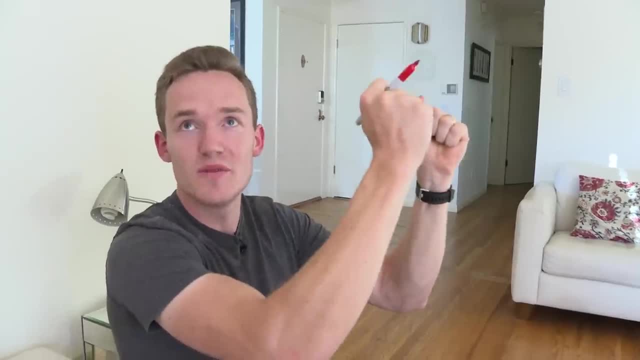 all the previous rational numbers and you say, hey, when are those two denominators going to fit in here? and then you add up the denominators and you say, hey, when are those two denominators going to add up to five? that's where I need to insert one, but it looks so much pure and pristine when we have this. 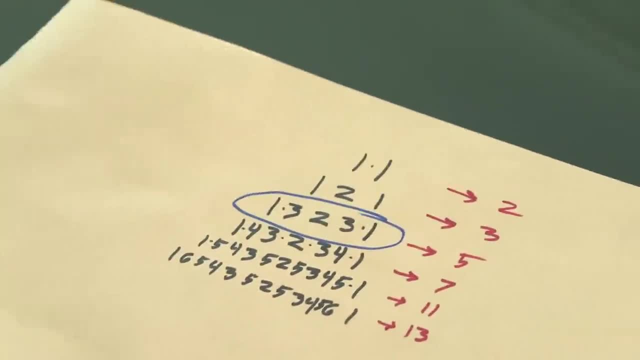 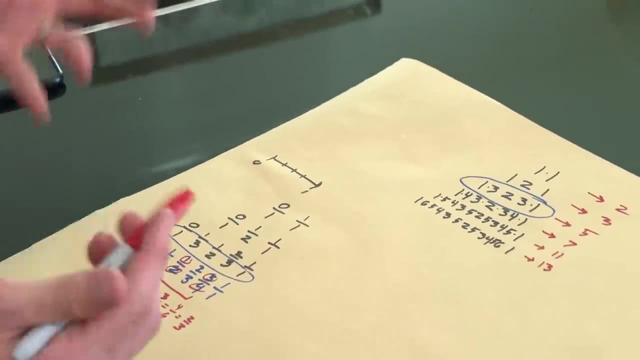 pyramid. and I don't mention that it's related to rational numbers. so you might say, oh, it's kind of a natural object, and if you think hard about when do certain rational numbers come up? the amount that you're adding has a lot to do with the 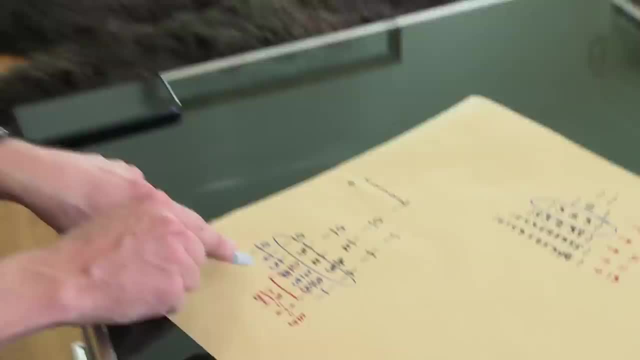 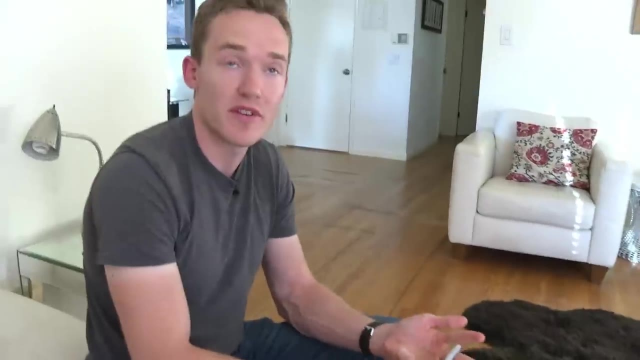 number of factors of that. for example, this next time when I'm adding one fifth, I actually know we're gonna get a lot more numbers because five we have to add one fifth, two fifths, three fifths, four fifths. none of those reduce, whereas it's not that we're gonna add one sixth, two sixths, three sixths, four sixths. 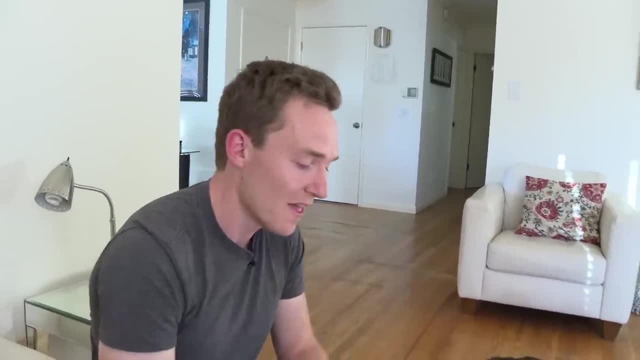 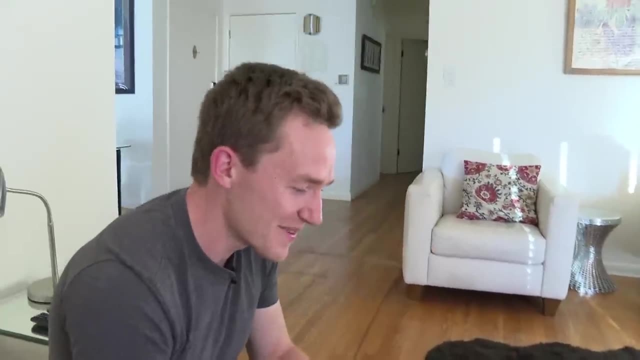 because two sixth has already accounted for, three sixth has always accounted for. so there's some, you know, loose connection to the idea of how divisible is the next number and things like that. priminess is in there, right, so we might expect. so the million-dollar question, yeah, does this thing keep spitting out? 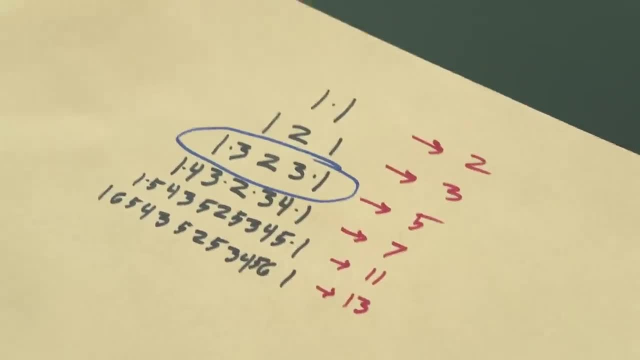 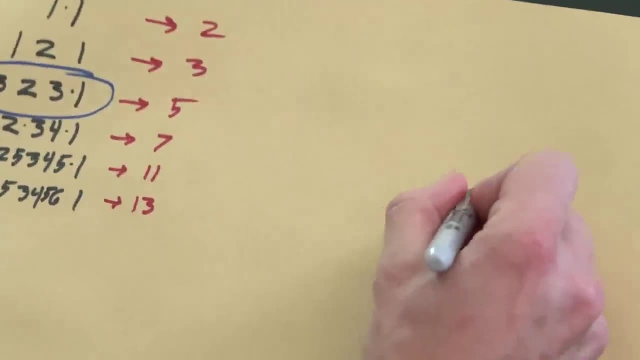 prime numbers. sadly, the pattern actually breaks and there's a there's a little hint to when it breaks too, so I'll do a couple more rows. we should expect that we need to insert numbers corresponding to one seventh, two sevenths, three sixths, two sevenths, three sevenths, four sevenths. all of these, because none of these. 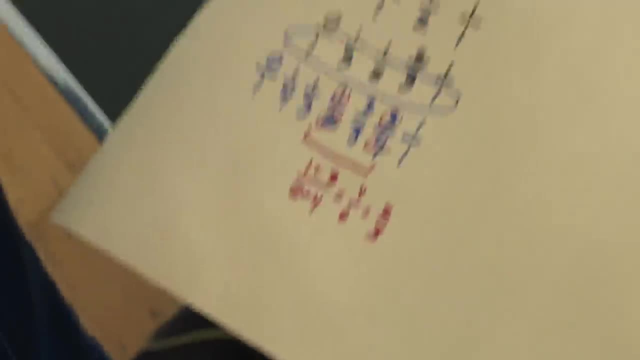 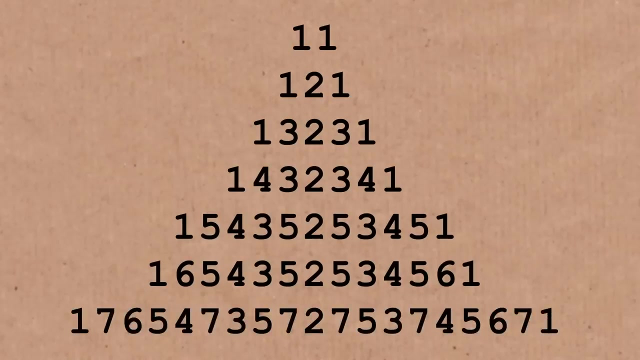 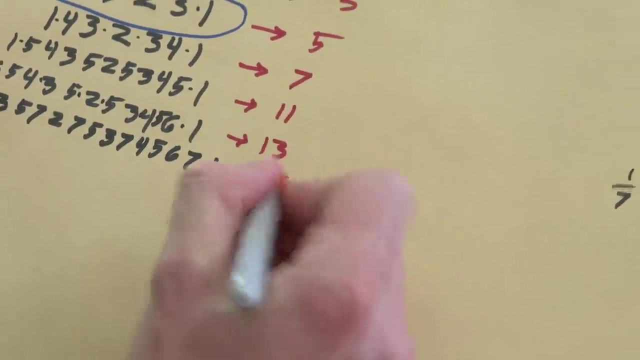 fractions reduce, I'm expecting. so you're using what we learned there, yeah, to help guide you here. I know that I'm gonna be inserting six different sevens basically, and so this is now interesting. we count how many are there we've got. we should know it's gonna be 13 plus 6, so on the one hand, the pattern continues, but on 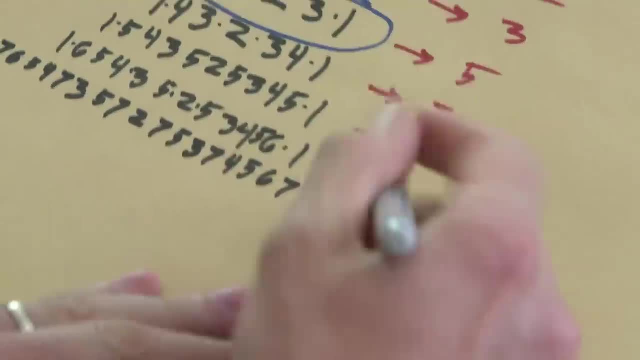 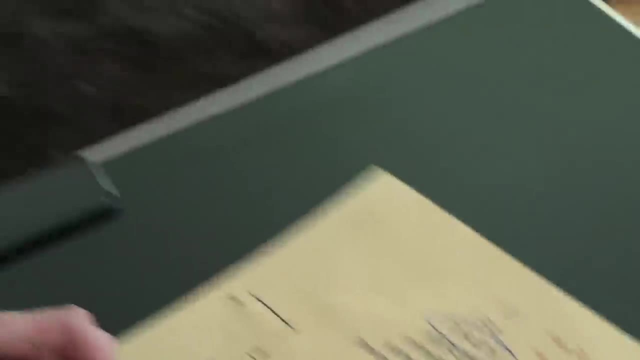 the other hand, you know there's a little chink in the armor because 17 is sitting here, just kind of sitting there, and I'm not sure if that's the right way to do it. I'm kind of wondering why it's been left out of the club. yeah, this is a. this is a. 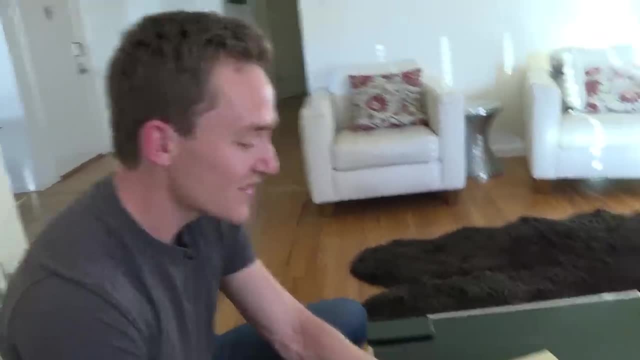 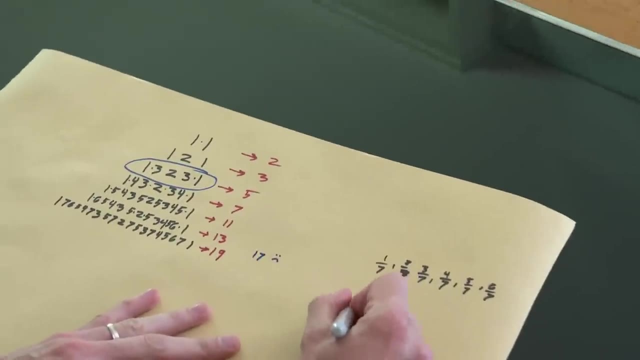 worrying sign. it's a worrying sign, but it does actually continue. the faster way to do this, rather than inserting them all like this. I can now ask you know how many eighths are we gonna be adding? how many reduced fractions are there with an eight and the reduced fractions with eight are basically just all the odd. 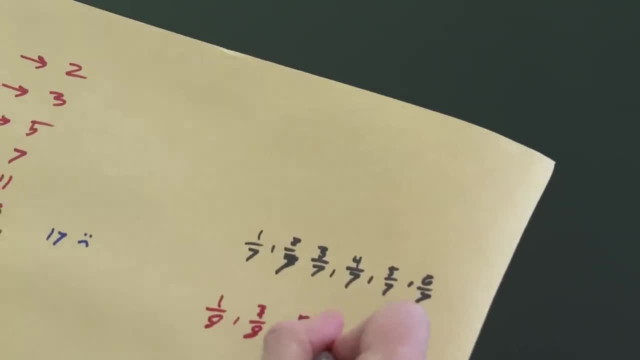 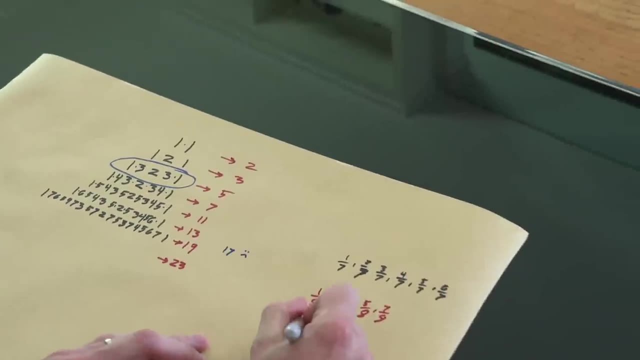 numbers. so there's four that I should be adding, so I kind of know that the next one is gonna get me to 23, regardless of how many I insert in there, and then nine. so one-ninth, two-ninths, three-ninths is not reduced, but four-ninths, five-ninths, 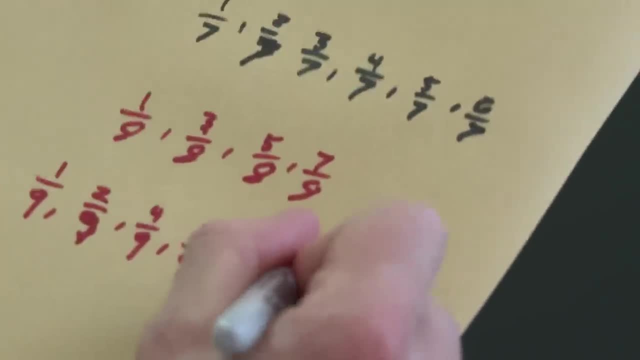 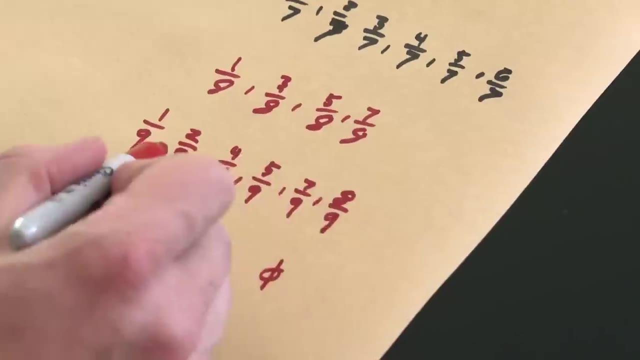 six-ninths is reduced so I won't include it. seven-ninths and eight-ninths- people who are curious? the number that we're counting here, all of the basically numerators that don't share any divisors with the denominator would be called the. 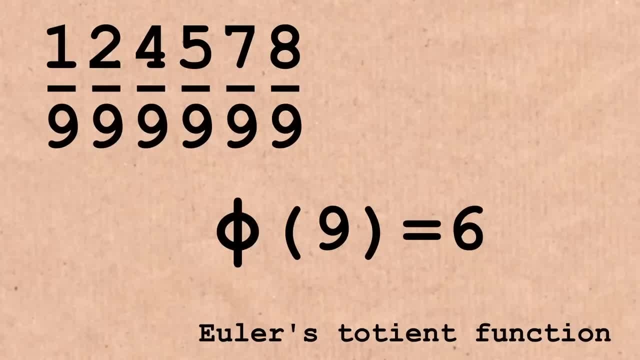 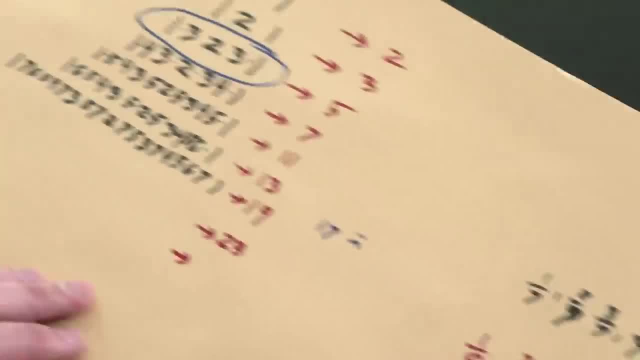 Euler-Tosch function of your number nine and that's basically counting. how many numbers are there like this? numbers less than nine that don't share any factors with it. so here we know that we would be adding six and that gets us to 29, which 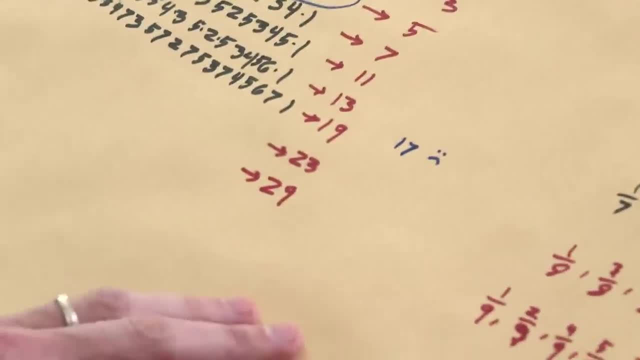 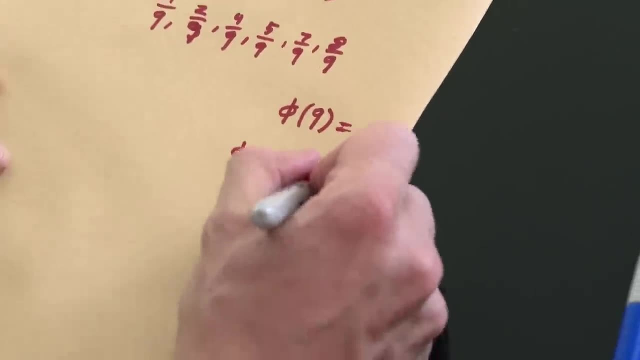 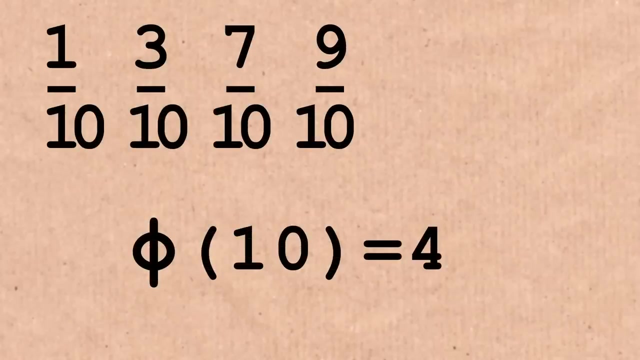 again feels pretty good. and then, in terms of ten, you know the Euler-Tosch function of ten saying hey, how many numbers up to ten don't share any factors with it, it's actually only four. you can see this with one tenth. two tenths isn't good, three tenths is good, four tenths no good, five tenths: no good. 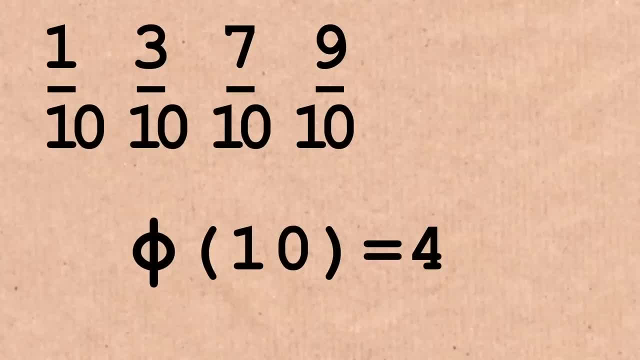 six tenths. no good, all of those reduce seven tenths and nine tenths. these I kind of know this because these are the last digits you would expect of prime numbers. all the other, there's only four digits available. so if we add four to this, that's when. that's when it properly breaks. it broke. yeah, it properly broke. 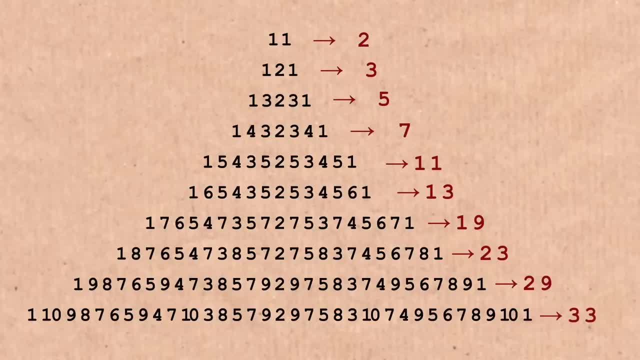 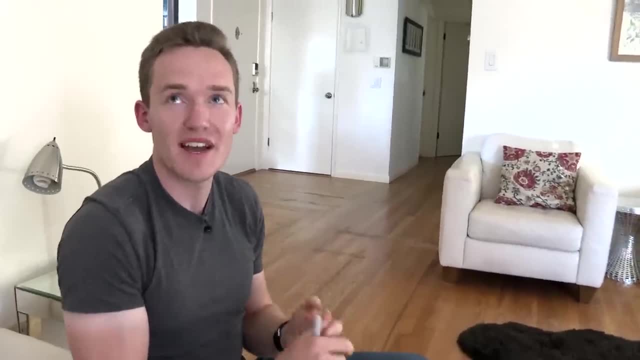 properly broke. and in this case- you know, in our previous example, we could do a little bit of analysis to say: oh well, you know, it was necessarily indivisible by two, three and five. so there's a good reason, as far as I can tell. this is just. 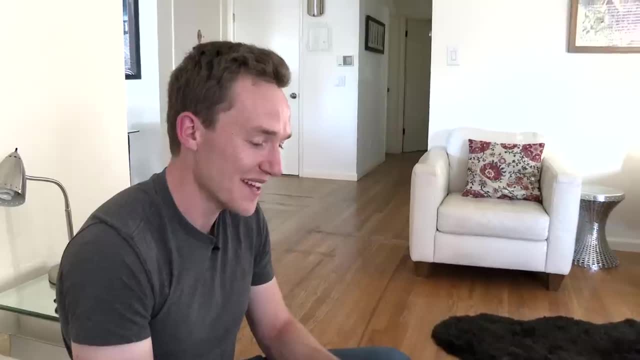 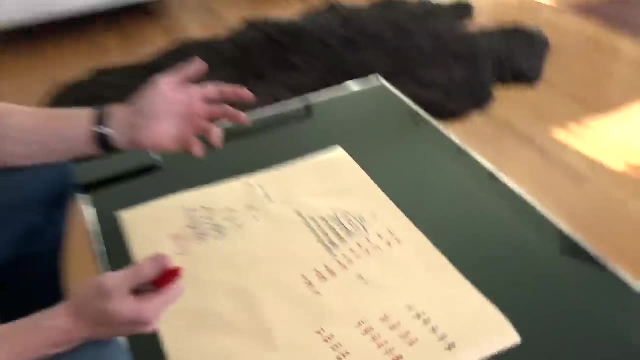 a meaningless coincidence. this is a good example of Richard Guy's strong law of small numbers, because as we go through these first few numbers, we can have a little bit of a sense that there's a likelihood they'd coincide with primes, because it starts with two and then you add one to it, and thereafter you're always adding an even. 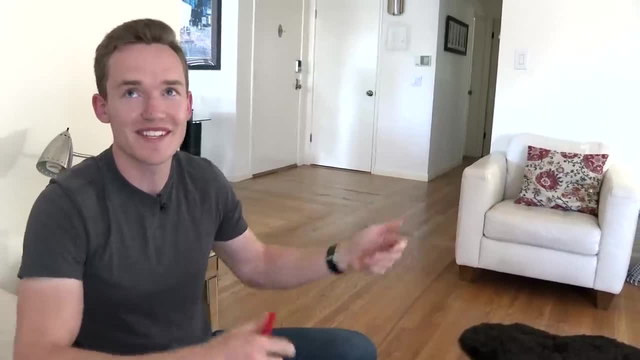 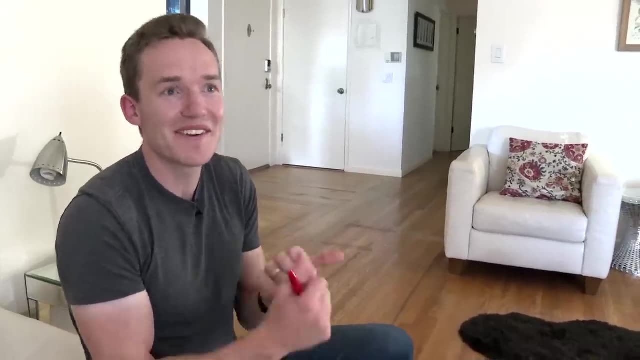 number. so you're either, you know, typically adding a two or four, maybe a six in there, and so you're getting things that are odd. and so, if you think of it as a probabilistic process, you're kind of guaranteed not to hit any even numbers. so that gives you a little something. and when the numbers are so 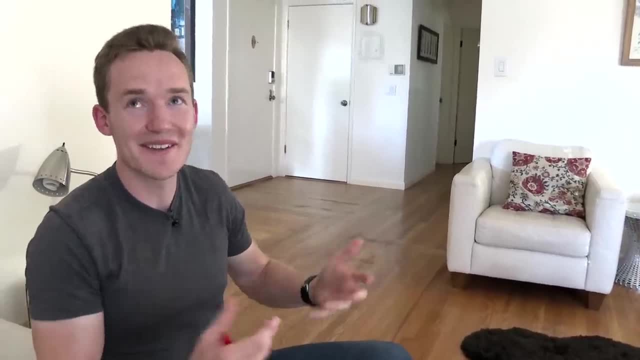 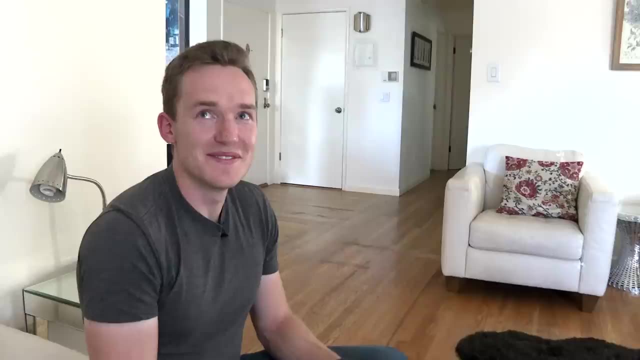 small. if you're an odd number, you know it's my guarantee that you're going to get a bigger prime, but it's more likely. it's like 50. more likely you will be. so we're playing around in this part of the number line where the primes 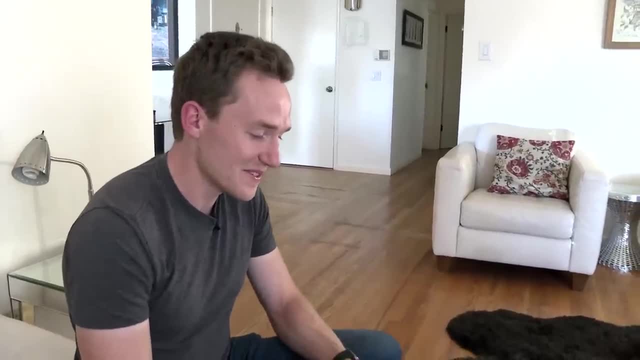 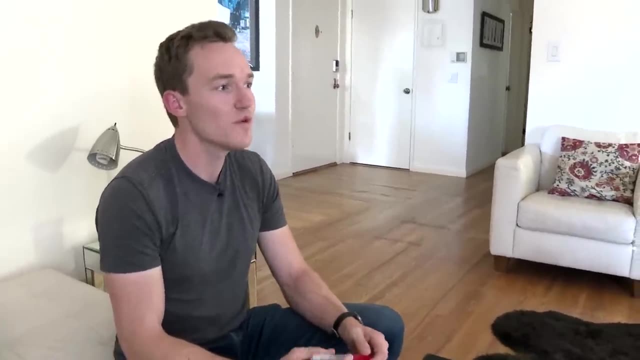 are still pretty dense, exactly, yeah, and so you're likely to see these sorts of patterns that, um, just they just don't hold that long. there's plenty of things like this, actually, where I think, when we do pencil and paper intuition building, it's common to just deal with smaller numbers. and you know the thing that 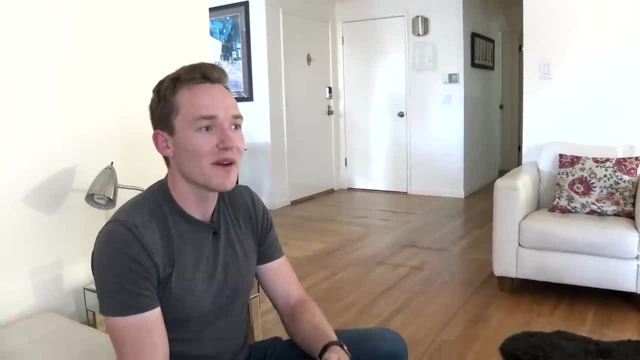 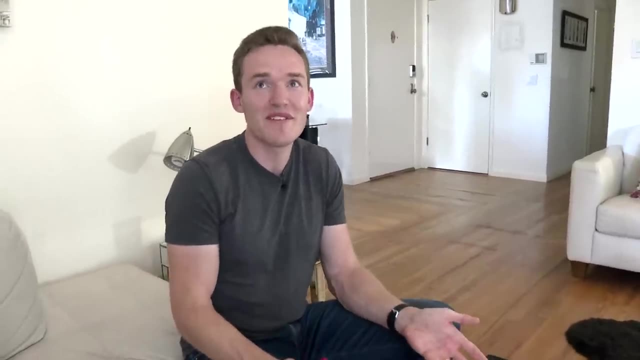 someone might want to take away is understand. is there a way that small numbers are not representative of the larger numbers and, for instance, how many primes are there between zero and 100? it's about 25% of them. that's a very atypical part of the number line. right, because you go? 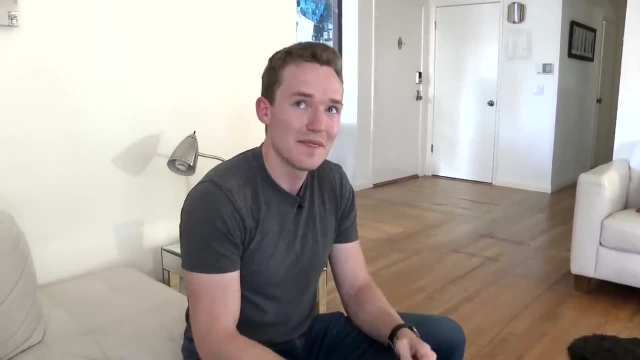 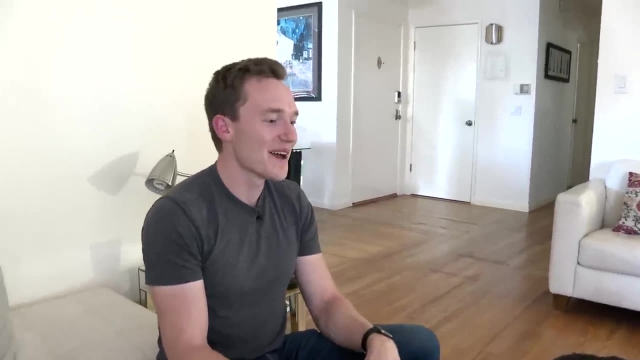 out to any other part and it's many fewer that are there. it's like if you watch Hollywood movies you would think everyone on earth is really good looking. exactly, yeah, yeah, if, if prime numbers are like the sexiest numbers available, right, that part of the number line right towards the beginning, that is.